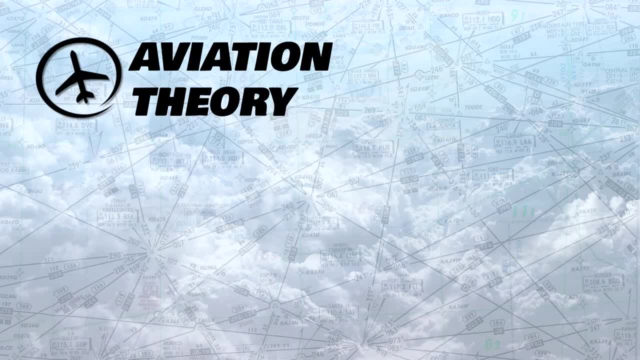 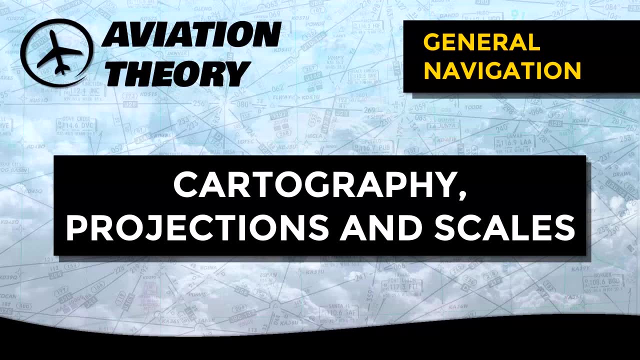 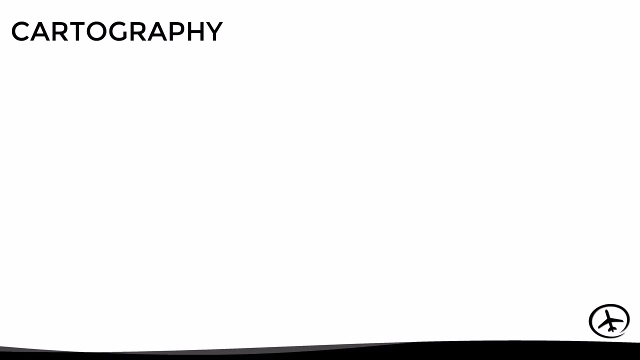 Today we will talk about cartography, projections and scales, which are essential concepts for the proper interpretation of navigation charts. So let's start by defining cartography. This word comes from karto, which means map, and graph, which means write, and it is the 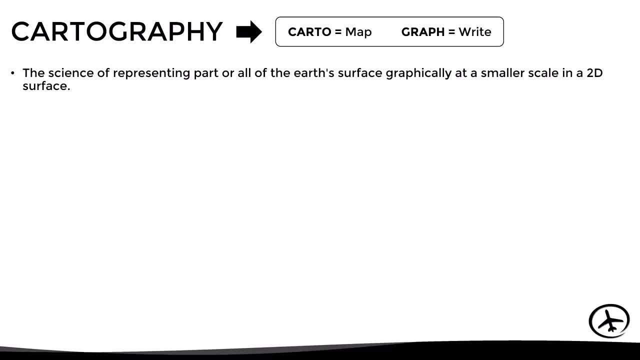 science of representing a part or all of the Earth's surface graphically at a smaller scale. in a 2D surface such as a piece of paper, This graphic representation obtained is called a map. But why do we sometimes say map and sometimes chart? Well, a chart. 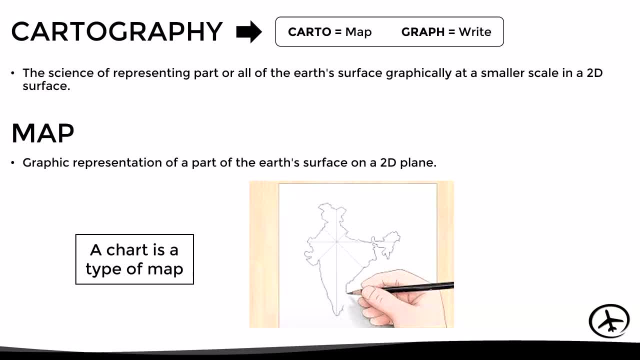 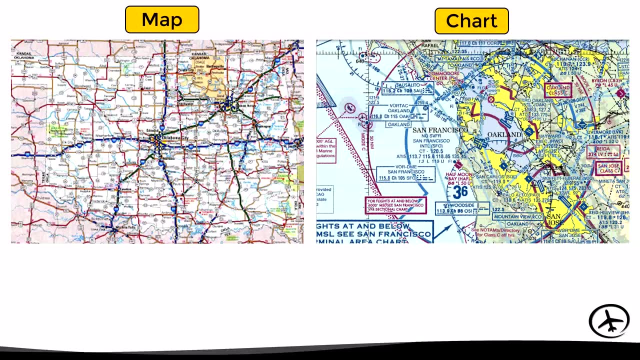 is actually a type of map. Let's look at this in more detail. In general terms, a chart is a specialized map which contains information related to a particular purpose. For example, a nautical chart will show information such as sea depth, lighthouses, etc. 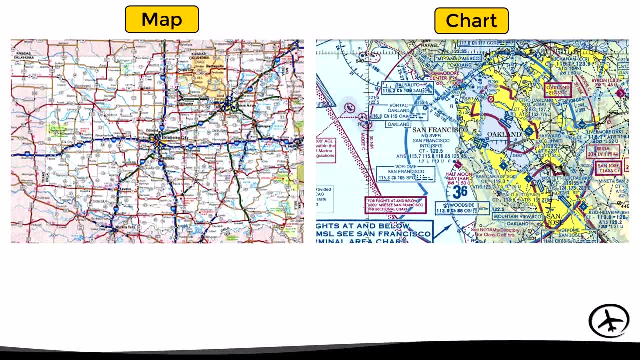 However, in the case of aviation, an aeronautical chart is a map adapted to the needs of air navigation, which contains detailed, relevant information on the most important aspects, such as obstacles, nav, aids, airports, airspaces, etc. Now, with this being said, when we try, 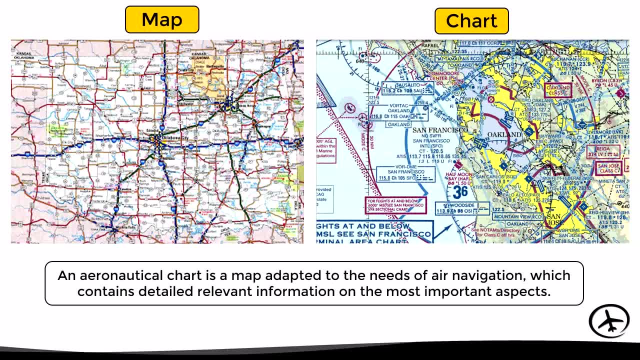 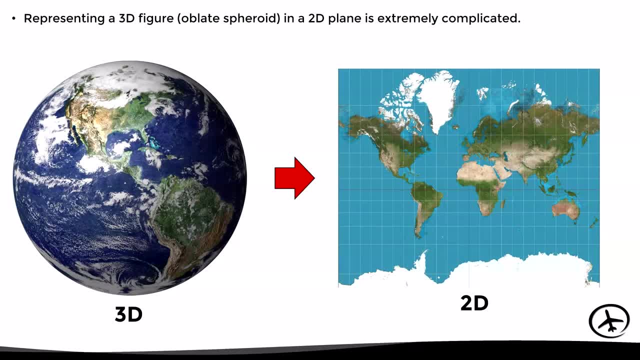 to create a map or chart that correctly represents the surface of the Earth, we run into a big problem, and it is that representing a 3D figure such as the Earth in a 2D surface is extremely complicated. Since it is impossible to represent the Earth on a 2D plane, maintaining 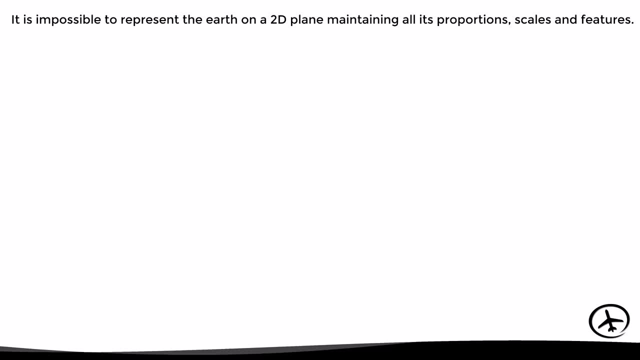 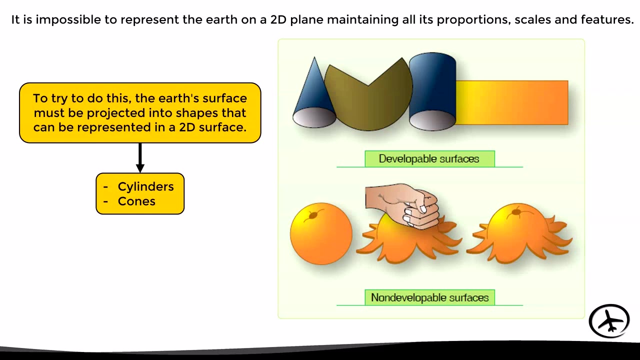 all its proportions, scales and features correctly. However, we can try to get as close to perfection as possible. To try to do this, the Earth's surface must be projected into shapes that can actually be represented in a 2D surface, such as cylinders or cones. 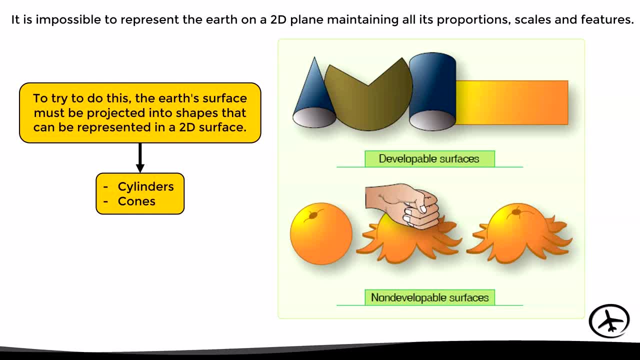 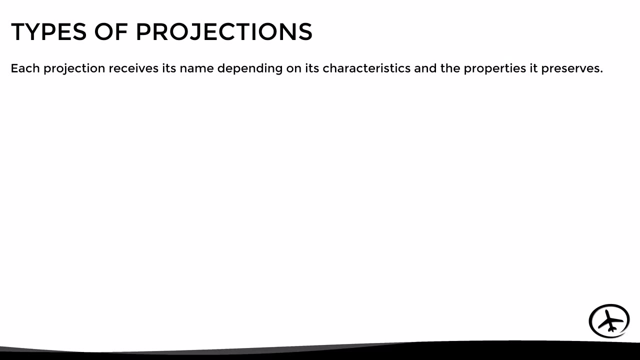 which are developable surfaces. Now, all these attempts to represent the Earth in different shapes are known as projections, and there are a lot of them. Each projection receives its name depending on its characteristics and the properties it preserves. For example, a conformal projection maintains the correct shape of objects and surfaces. An equivalent 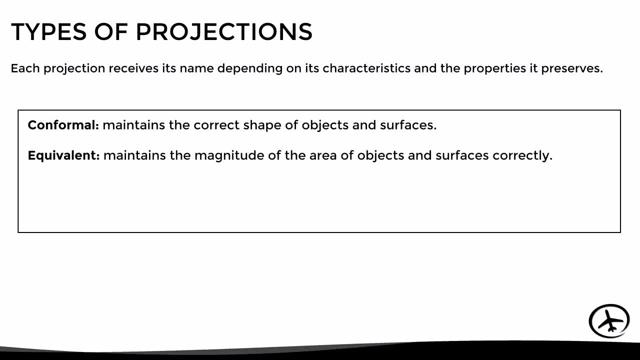 projection maintains the magnitude of the area of objects and surfaces correctly, An equidistant projection maintains the ratio of the distance between two objects or surfaces correctly, And an azimuthal projection maintains the direction between two objects or surfaces correctly. Now, although it would be great to be able to include all of these features, 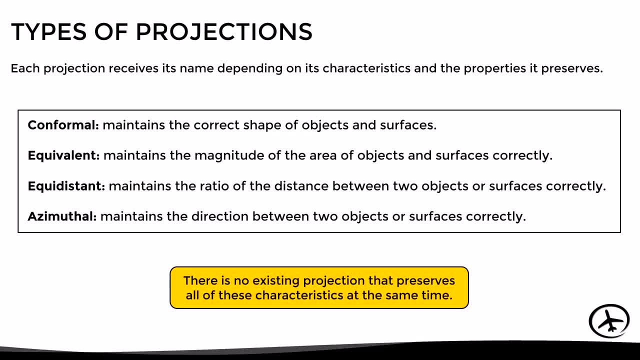 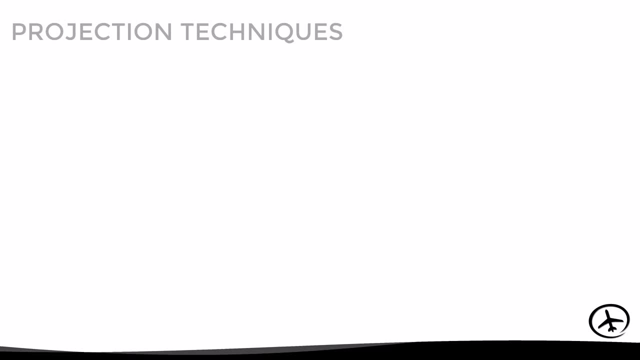 on the same map. there is no existing projection that preserves all of these characteristics at the same time, So it must be decided which of these features is more important to include in the map, depending on the shape of the Earth. Now, to understand better how a projection is developed, it can be described as putting 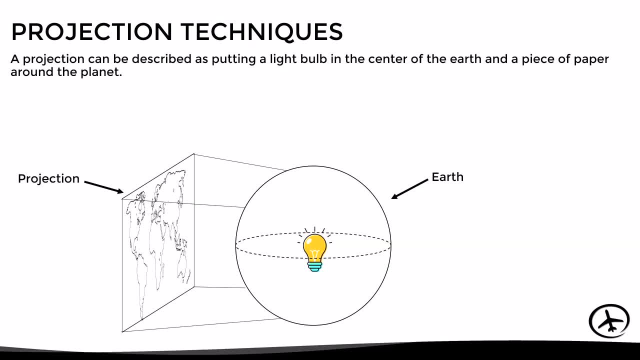 a light bulb in the center of the Earth and a piece of paper around the planet. Then, when the light bulb is turned on, the surface of the Earth is projected onto the piece of paper, becoming a map. This way, the resulting map will depend on how the paper is placed. 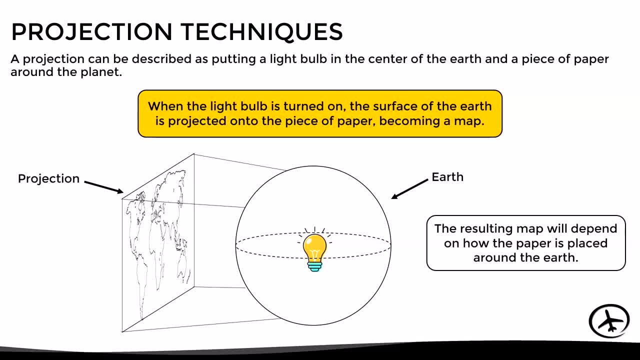 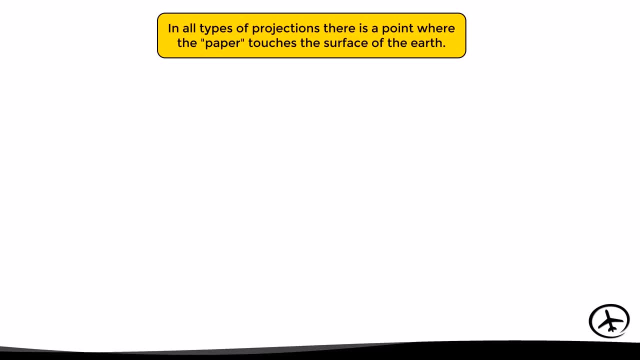 around the Earth, and that is why there are different types of projections. Now, an important thing regarding this: The most common use of a projection is that in all types of projections, there is one or more points where the paper touches the surface of the Earth, and, as a general rule, these 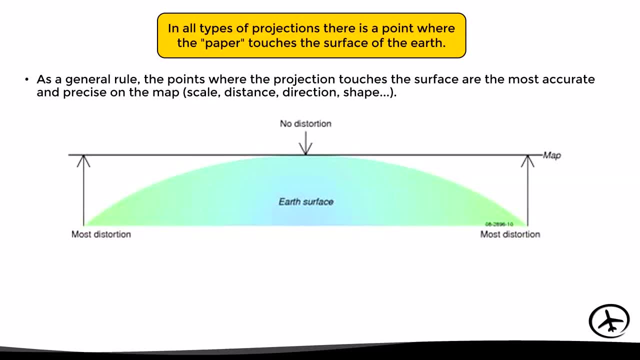 points where the projection touches the surface are the most accurate and precise in terms of scale, distance, direction, shape, etc. and as we move away from these points, the map begins to distort. So, with this being said, let's take a look. 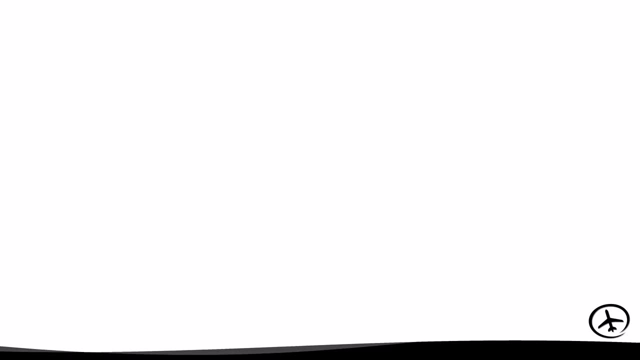 at the most commonly used projections, starting with the azimuthal projection. It consists of a flat surface, a flat surface and a flat surface. The azimuthal projection is a projection which is a flat piece of paper that touches the Earth at one of its poles, as we can see. 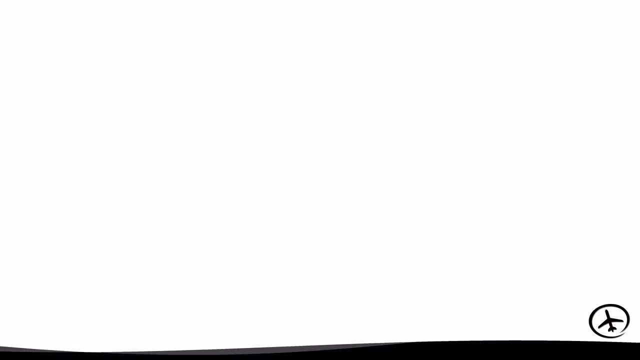 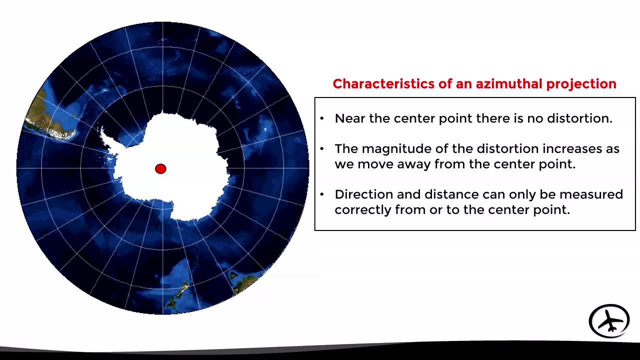 in this images. The main characteristics of an azimuthal projection is that near the center point there is no distortion. the magnitude of the distortion increases as we move away from the center point, and direction and distance can only be measured correctly from the center point. This projection is often used to map the poles, but is not commonly used for navigation. 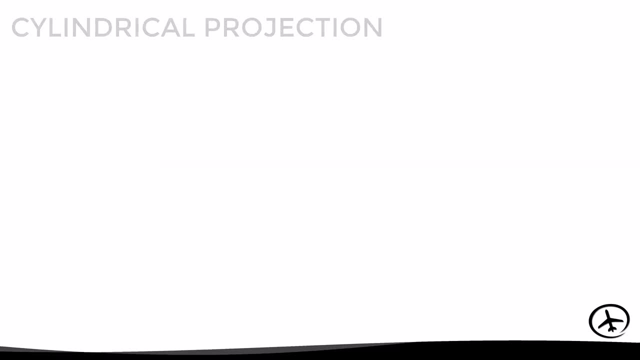 Now the next one is the cylindrical projection. This projection is often used to map the poles, but is not commonly used for navigation. Now the next one is the cylindrical projection. The next one is the cylindrical projection, which consists of a piece of paper that is 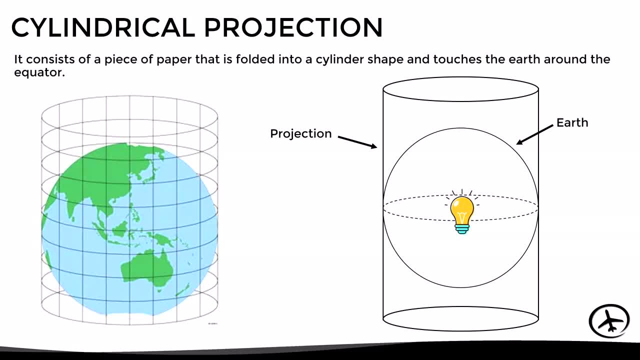 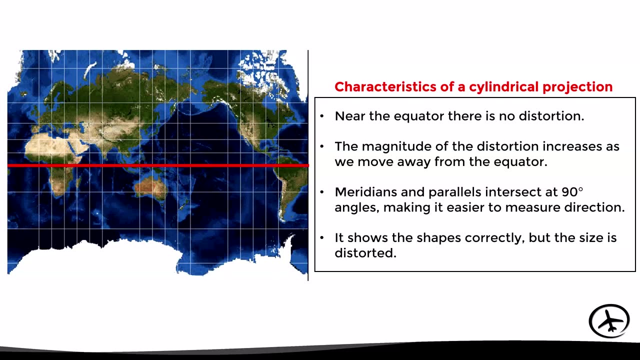 folded into a cylinder shape and touches the Earth around the equator, as we can see in these images. In this case, the projection touches the Earth around the entire equator line. Therefore, the main characteristics of this cylindrical projection are that near the equator there is no distortion. the magnitude of the distortion increases as we move away. 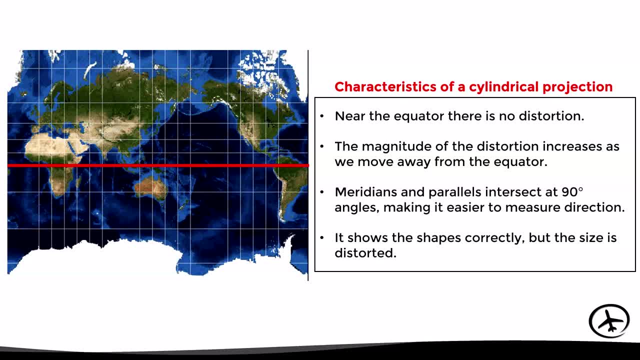 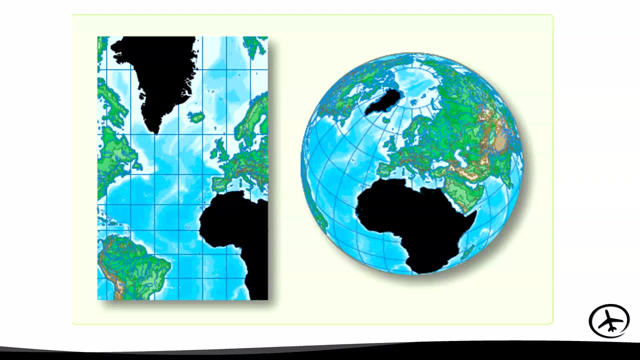 from the equator and parallels intersect at 90 degrees angles, making it easier to measure direction, and it shows the shapes correctly, but the size is distorted. a clear example of this is the representation of africa and greenland. here we can clearly see that in reality, africa is much 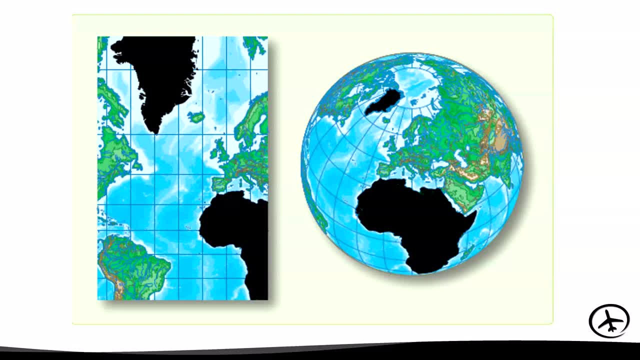 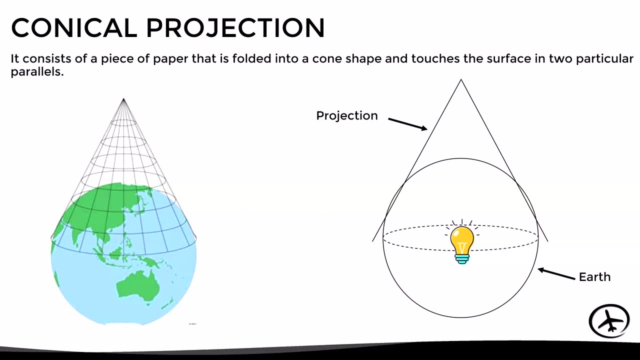 bigger than greenland. however, because of the distortion of this cylindrical projection, it looks like it is almost the same size. finally, there is the conical projection, which consists of a piece of paper that is folded into a cone shape and touches the surface in two particular parallels, which are known as standard parallels, as we can see in these images. in this case, since 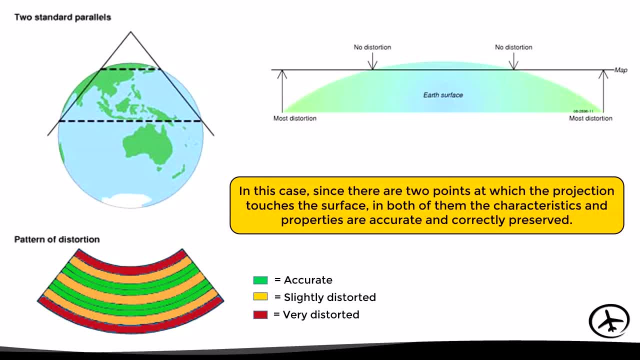 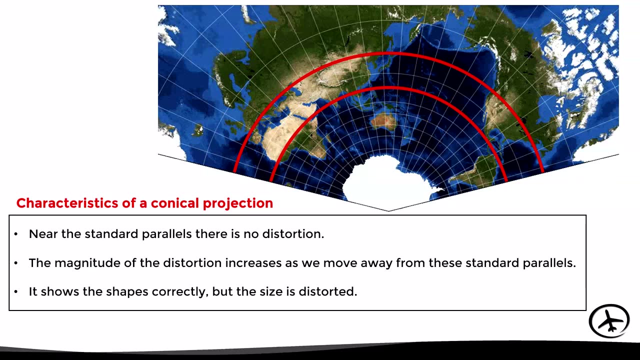 there are two points at which the projection touches the surface. in both of them, the characteristics and properties are accurate and correctly preserved, giving, as a result, this pattern of distortion. now, the main characteristics of this conical projection are that, near the standard parallels, there is no distortion. the magnitude of the distortion increases as we move away from these. 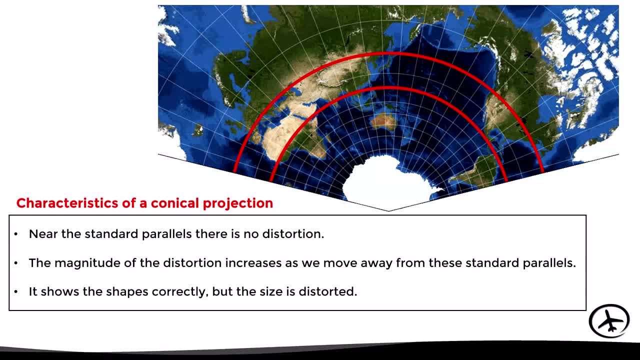 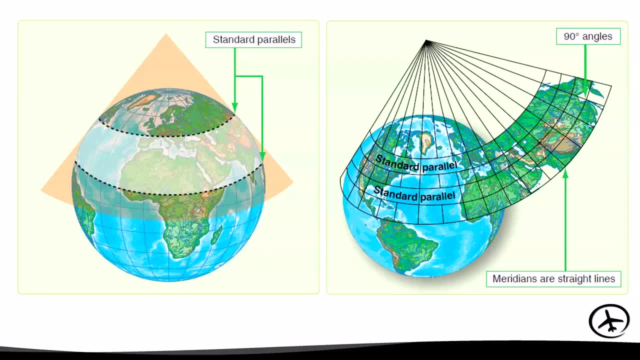 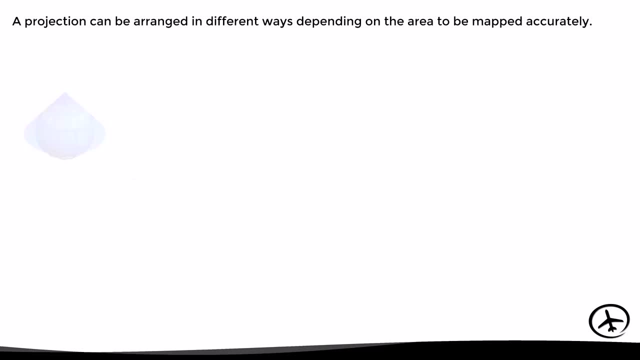 standard parallels and it shows the shapes correctly, but the size is distorted, just like in the cylindrical projection. here we can see an example of how a map is developed using this conical projection. finally, something important to mention is that a projection can be arranged in different ways depending on the size of the projection. the size of the projection can be: 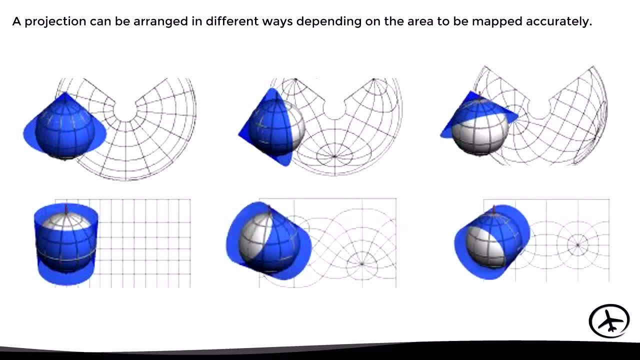 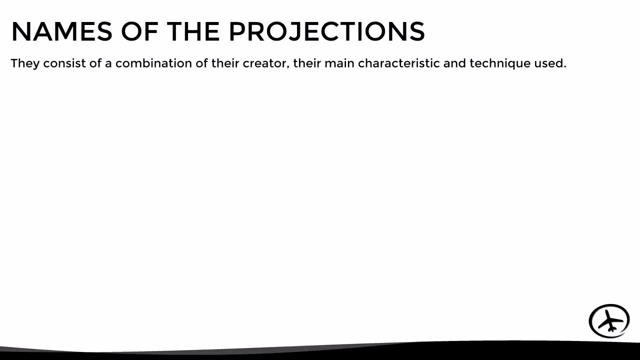 arranged in different ways depending on the area to be mapped accurately, as we can see in these examples. now, regarding the names of the projections, they consist of a combination of their creator, their main characteristic and technique used. for example, the most used projections for navigation are the lambert conformal conical and the mercator conformal- cylindrical. 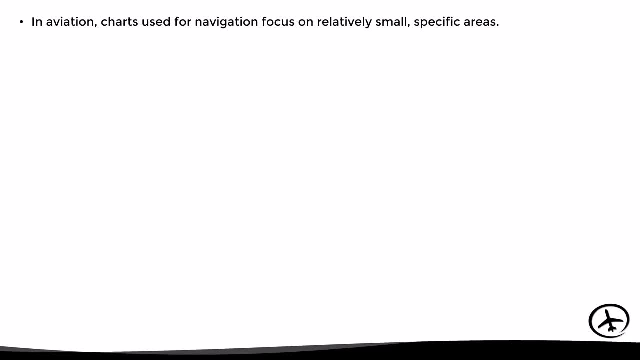 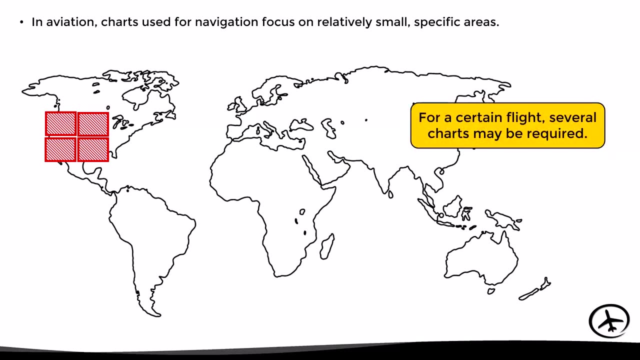 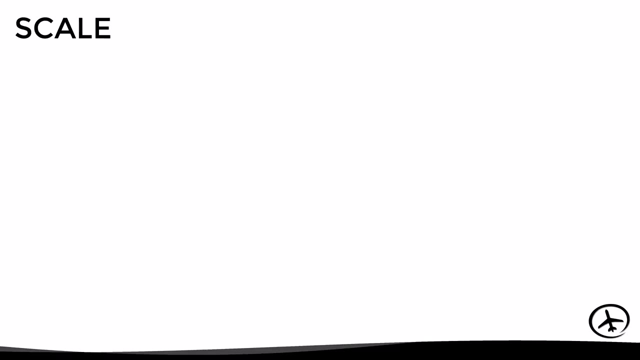 in these cases, to avoid excessive distortion. the charts used for air navigation focus on relatively small specific areas and therefore for a certain flight, several charts may be required. let's now move on to the scale. on an aeronautical chart, it is important that the proportions of 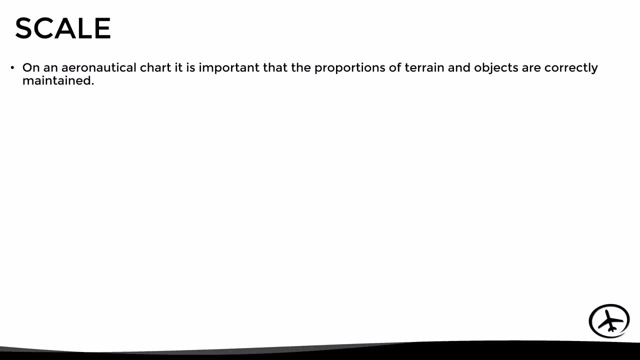 terrain and objects are correctly maintained and the scale is the relationship between a measurement on the map or chart and the actual measurement on the earth, and its formula is very simple: it is real distance divided by the map distance. and the scale is very simple: it is real distance divided by the 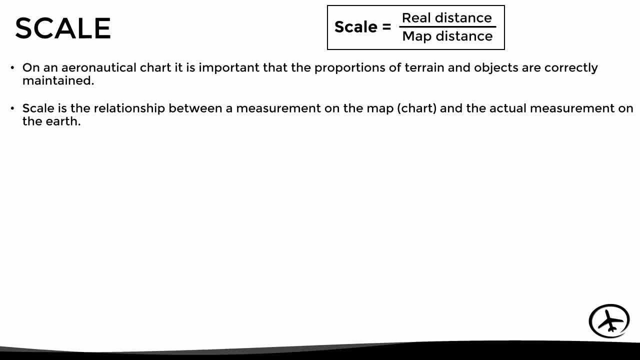 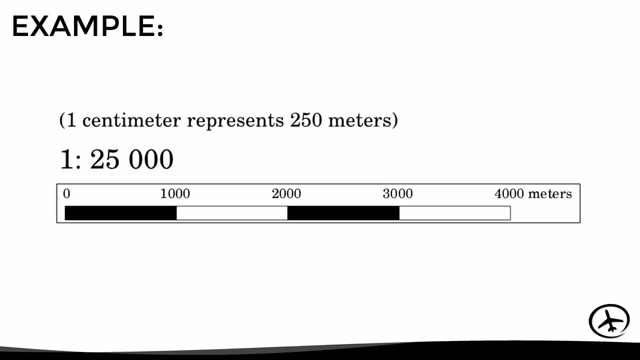 map distance. now, all maps publish the scale with which they were designed, and this can be found in different formats. for example, they can publish a numerical scale or a graphic scale or even a plain text scale. here we can see some examples of how the scale is published on a map. this information 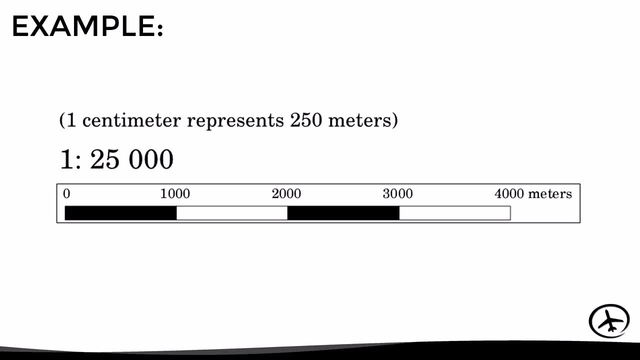 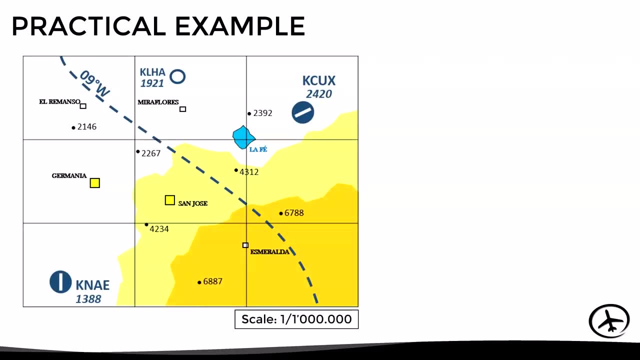 is really useful when we have to determine distances on a map without a plotter. let's see an example of how to do this. let's say we have this chart with a scale of one in one million and we want to determine the distance between the towns of germania and miraflores. however, we don't have a plotter, so 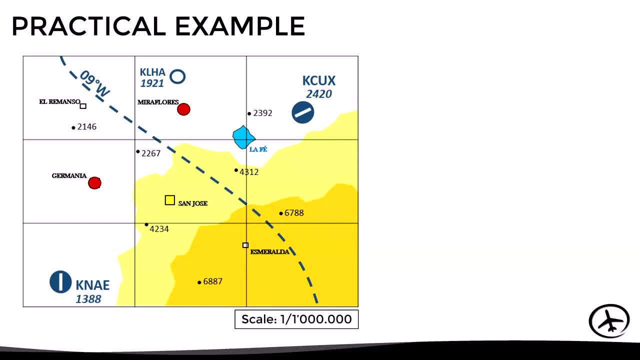 we have to use a regular ruler that measures centimeters. according to this, we measure a distance on the map of 16 centimeters. so now the question is: with this information, how can we determine the real distance between these towns? well, we have to use the scale formula. 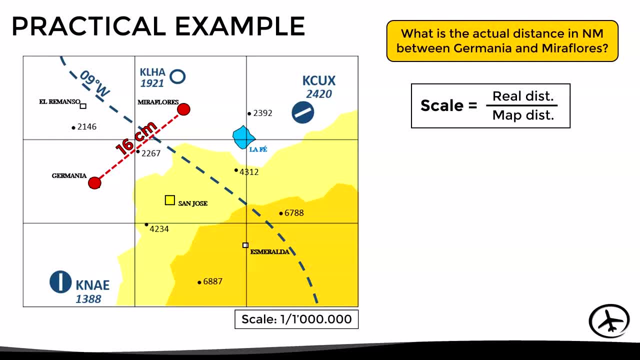 real distance divided by map distance. right now we know the scale and the map distance, so we just have to rearrange the formula to determine the real distance, which in this case is 16 million centimeters. with this we already know the real distance, but it is in centimeters, so we must. 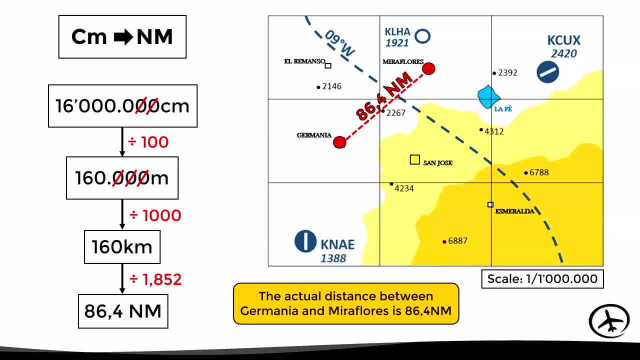 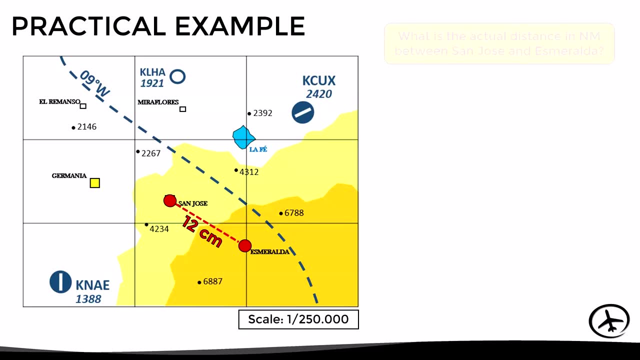 convert units to nautical miles, obtaining as a result a distance of 86.4 nautical miles. in this example, we used a map with a scale of one in one million. let's see now another example, but now with a scale of one in 250 000. in this case, we want to determine: